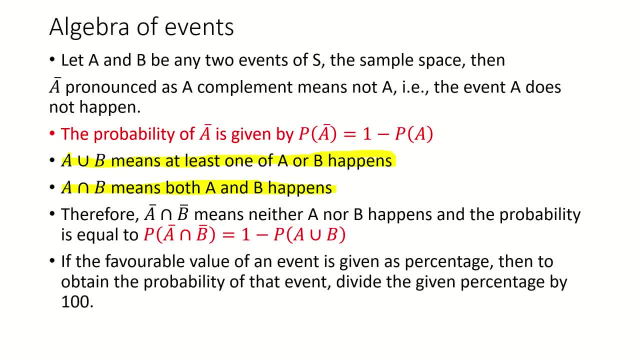 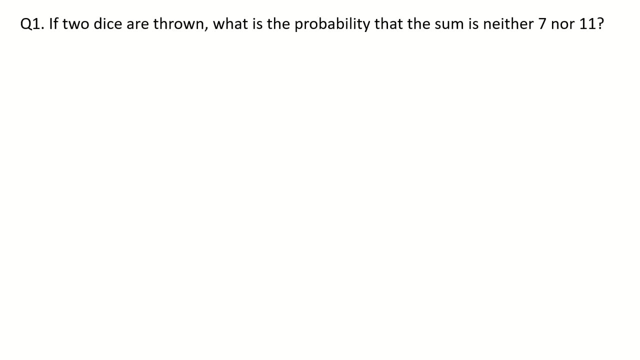 Of an event is given as percentage, then to obtain probability of those events you have to divide the percentage by 100. like, for example, if your event is given as 20%, then the probability of that event will be 20 by 100.. Now see the first example. 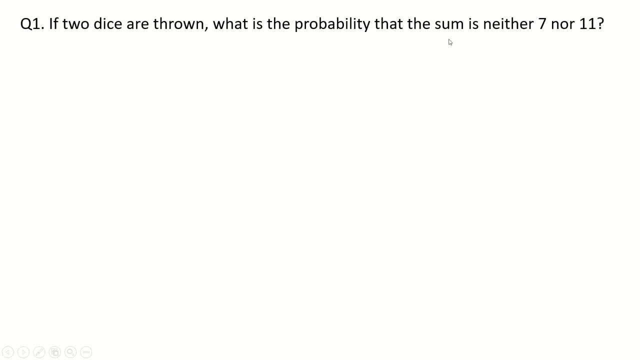 If two dice are thrown, what is the probability that the sun Is neither 7 nor 11? so whenever you get questions like this- neither 7 nor 11- so you always look for the positive event. this is the negative event, right like because, no, is there neither this nor this, so you look for the positive complementary event. the positive complementary event will be cut. this neither and nor. 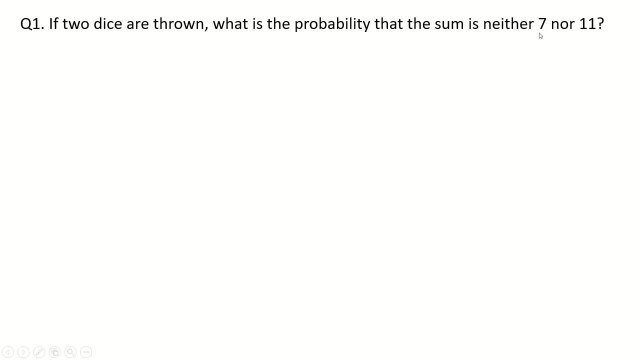 So the positive event will Be: sum is 7 or 11. so there are two events. one is sum is 7, another sum is 11. so you write the two events and when two dice are rolled, then exhaustive number of cases is 36. 6 into 6, 6 from the first dice, 6 from the second dice. multiply you get 36.. 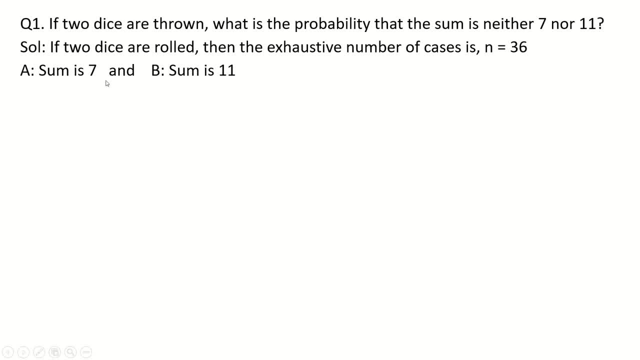 Now you Define the events: sum is 11, b sum is a, sum is 7 and b sum is 11. now what you are interested in: since you want the probability of neither 7 nor 11, that means you want the probability of a complement, intersection, b complement. a complement means neither 7 b complement means 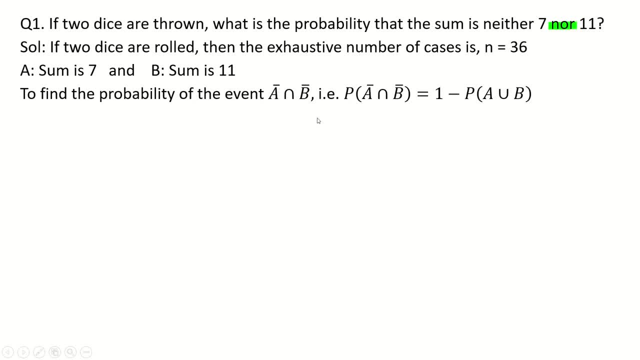 Nor 11. so you want this probability which is given by 1 minus a union. now you can find a union b very easily. first you find what is A is 1, 6. thus all the numbers which sum up to 7, all the numbers in a dice. now, number of elements in a is we denote it by n a? okay, there is number of elements.